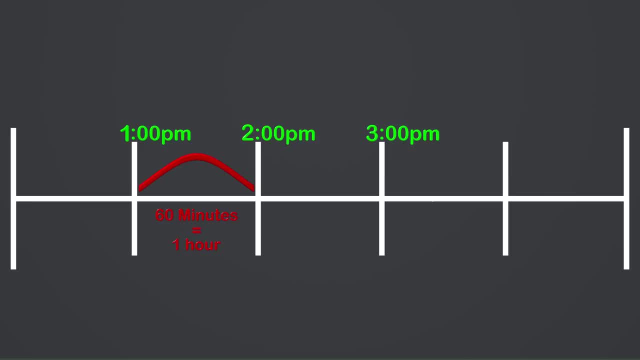 We can also break down the hour into smaller segments. It would take forever to draw 60 small lines in between each of these hours, so we will not use individual minutes. We can, however, start at half hours or 30 minutes. These lines represent 30-minute intervals or half hours. We can also break it down further into 15-minute or quarter-hour segments as well. 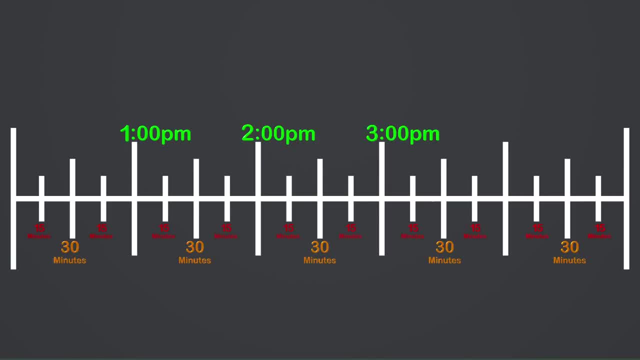 With this number line we can now see various numbers. With the number line we can now see visually how time has passed. For example, let's say I started playing games at 1.15 pm. I finished playing games at 2.30 pm. 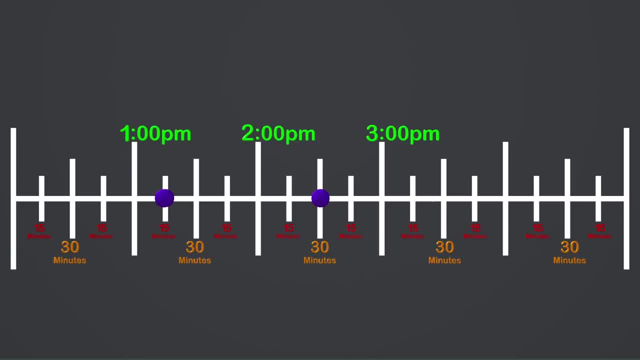 How long did I play games? By counting the amount of time from the start to the end on the number line, we will know how long I played games. One easy way to work this problem is to make jumps by the hour. So we start at 1.15 and jump 1 hour. 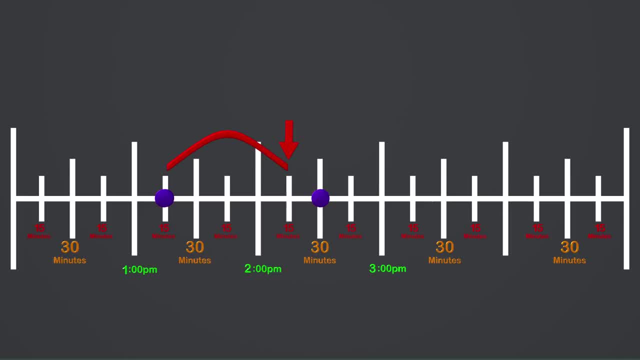 And that takes us to 2.15.. We now have jumped 1 hour, but we are still not quite there yet. We need to make one more jump. How many more minutes do we need to jump to make it to 2.30?? 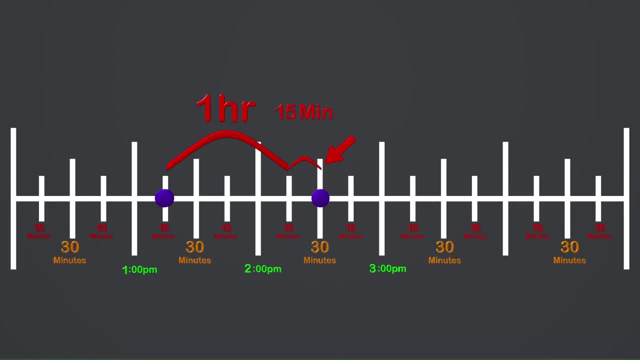 We need to jump 15 more minutes. So the total amount we jumped was 1 hour and 15 minutes. Great job guys. This is awesome. We just used a number line to solve a time problem. Let's bring in a word problem and see how the number line helps us. 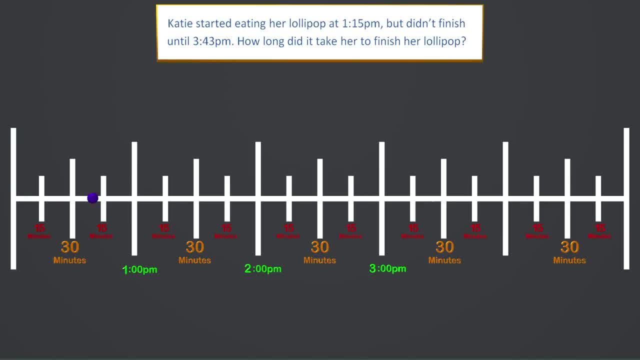 Here is a word problem that says Katie started eating her lollipop at 1.15 pm but didn't finish until 3.43 pm. How long did it take her to finish her lollipop? That must have been a huge lollipop. 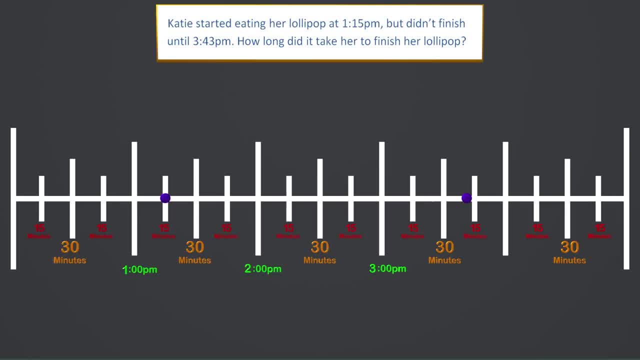 This problem can seem tricky, but once we start using the number line, we will figure it out. We start at 1.15. And move up an hour to 2.15.. Looks like we can still move another hour, so let's do that. 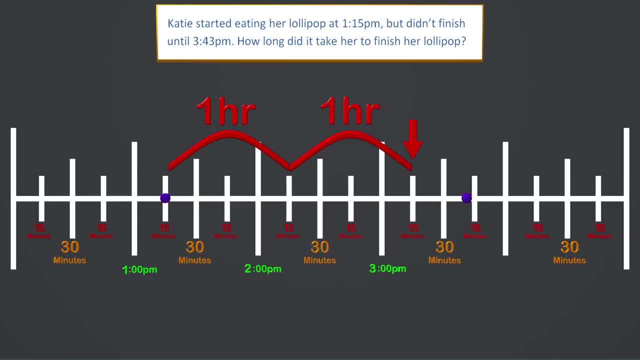 From 2.15 to 3.15 is another hour. We have moved 2 hours and that got us to 3.15.. But she did not finish until 3.43.. We need to figure out how many minutes are between 3.15 and 3.43.. 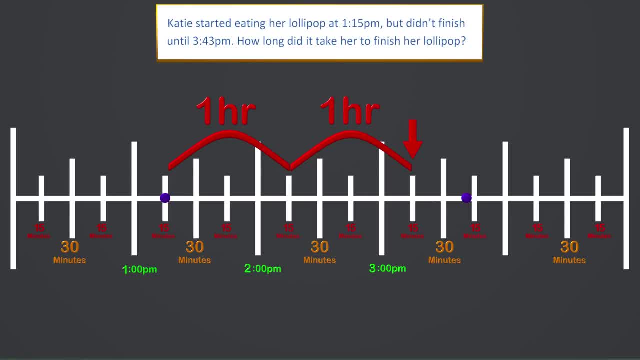 To do this. we are going to jump in smaller increments. We can go from the 15 here and jump 15 minutes. We are now at 3.30.. If we jump another 15 minutes, where does that put us? We actually jumped past where we need to be. 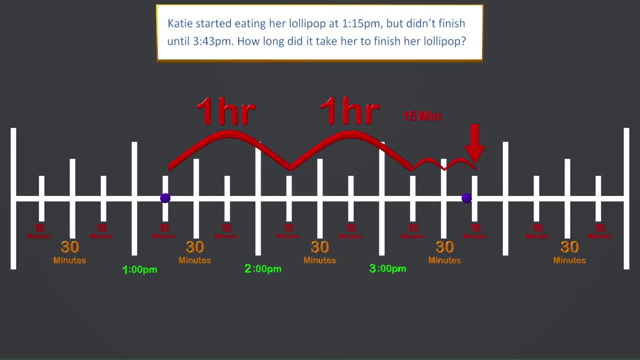 We are now at 3.45.. Let's erase this jump so we can learn how to make smaller jumps. We are back to 3.30.. And from here let's jump 10 minutes Now. we are at 3.40.. 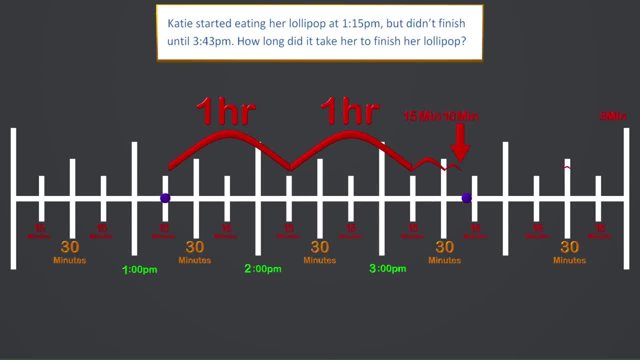 From 3.40, we only need to jump 3 more minutes. To finish the problem, we just need to add up the amount of jumps that we did. We jumped 2 hours, Then 15 minutes plus 10 minutes gives us 25 minutes. 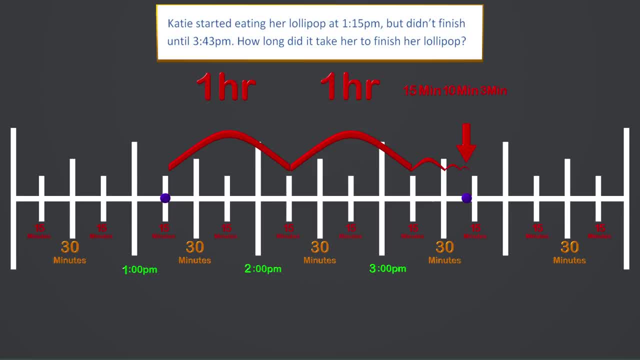 And the last jump is 3 minutes added to the 25 gives us 28.. So the answer is 2.40.. The answer is 2 hours and 28 minutes. That is how long it took Katie to eat her lollipop. 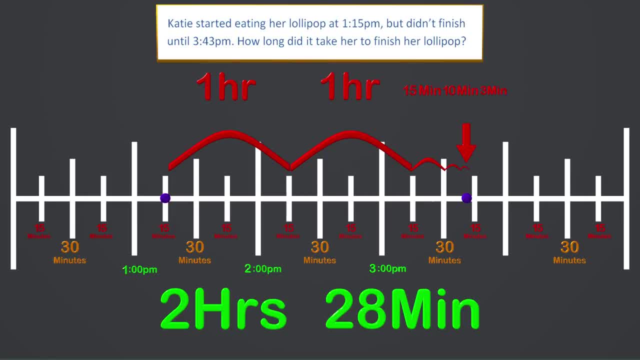 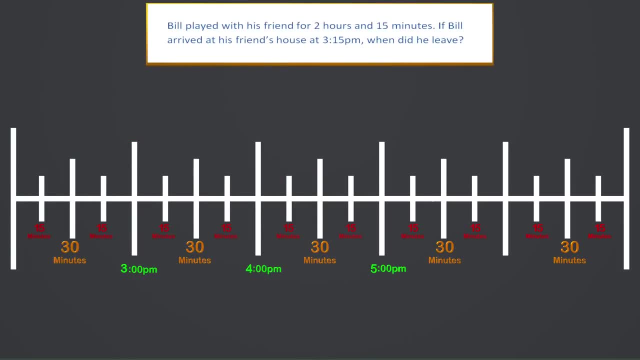 Great job, guys. Let's look at one more, using a number line again. Bill played with his friend for 2 hours and 15 minutes. If Bill arrived at his friend's house at 3.15 pm, when did he leave? 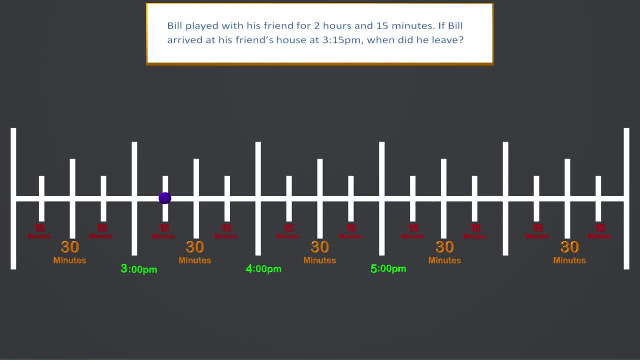 The problem tells us that Bill got to his friend's house at 3.15 and stayed there for 2 hours and 15 minutes, So we need to use the number line to add 2 hours and 15 minutes to see when he left. 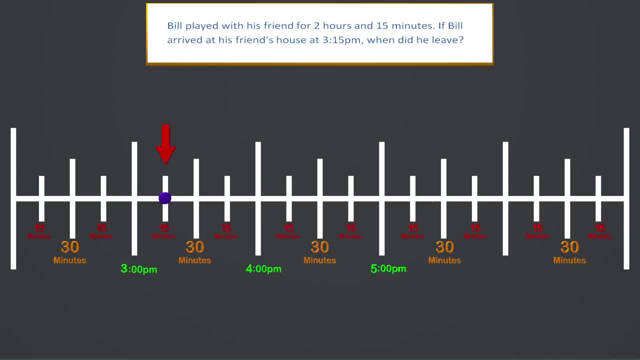 Here is the start: at 3.15.. We start by jumping with the highest increment we can, which is the hour. Let's jump 2 hours. We have jumped 2 hours and we are at 5.15.. Great job.